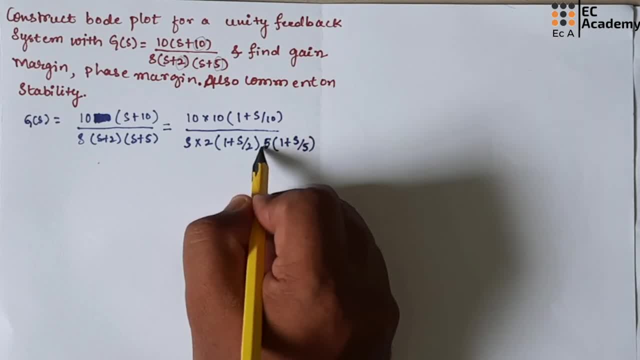 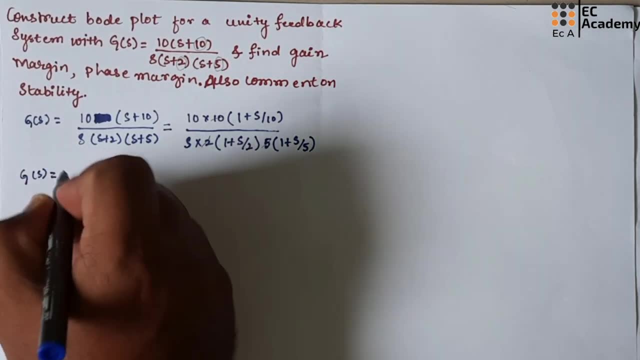 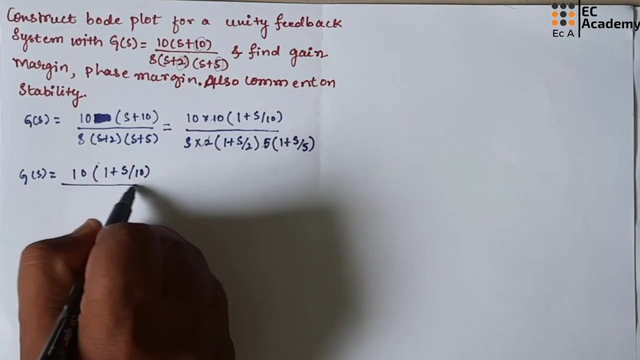 So here, 2 into 5, it is 10.. So 10 and this 10 we can cancel out, So we will left out with the transfer function. G of s is equal to 10 into 1 plus s by 10, whole divided by. 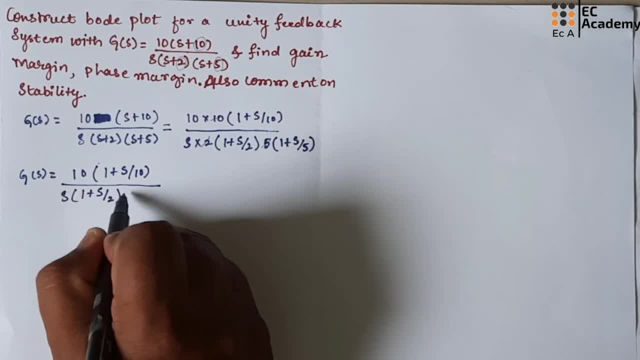 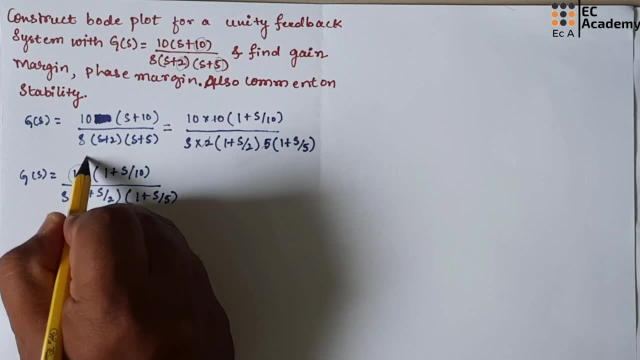 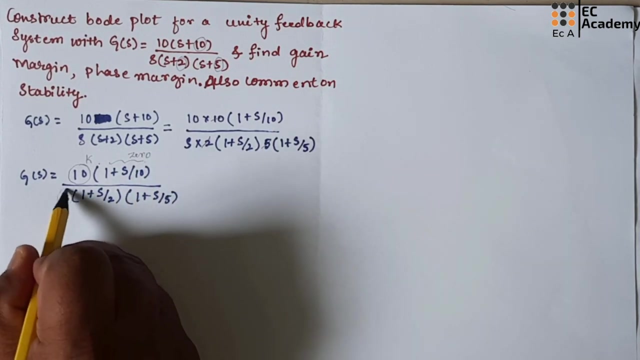 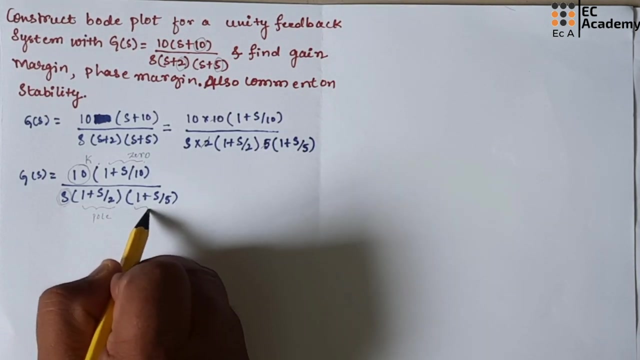 s into 1 plus s by 2, into 1 plus s by 5.. So this 10 represents constant k. This is one simple 0.. This is s that represents one pole at the origin. and this is one simple pole and this is another. 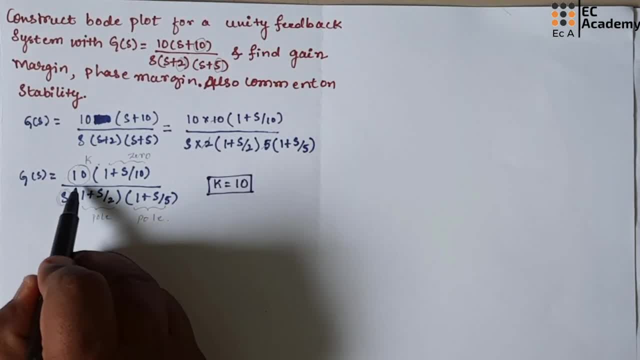 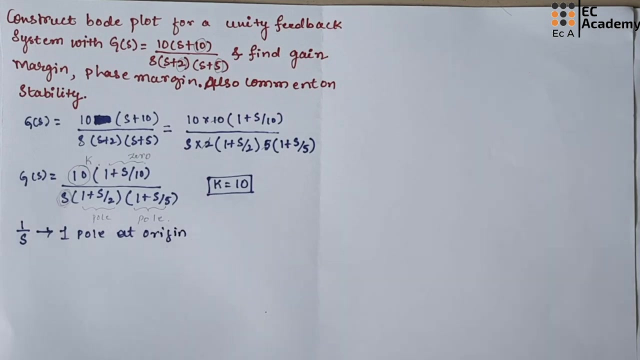 simple pole. So from this transfer function we obtain: k is equal to 10 and also there is 1 by s. Due to this, there will be one pole at origin. So this one pole at the origin will produce minus 20 dB per decade. 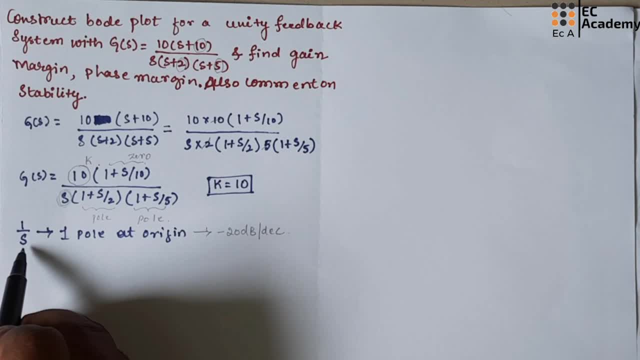 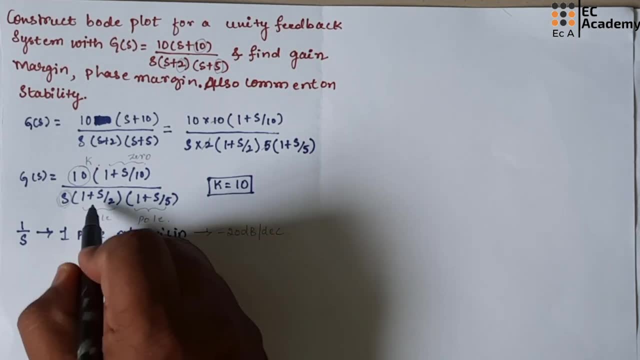 slope. If this term is 1 by s square, so which means there will be 2 poles at the origin, that will produce minus 40 dB slope. Then there is next term, which is 1 divided by 1, plus s by 2.. 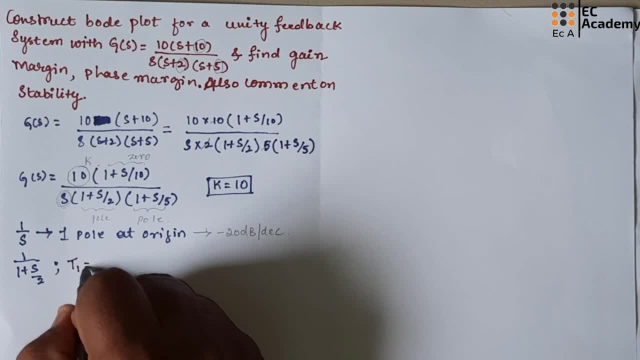 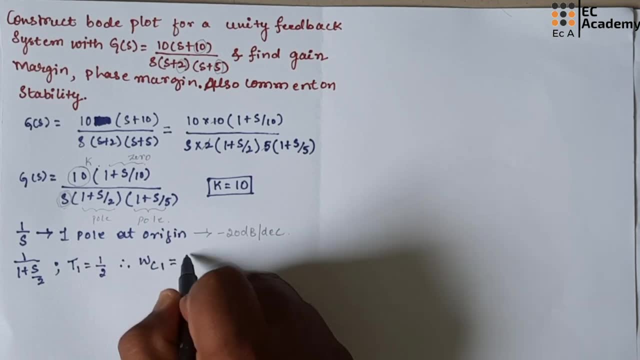 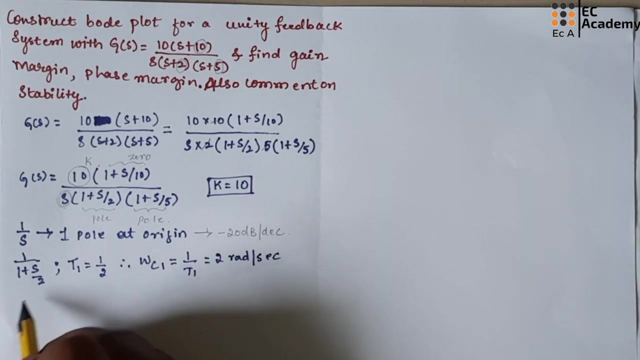 So, due to this, we can write: T: 1 is equal to 1 by 2.. Therefore, we can write the first corner: frequency: omega c1 is equal to 1 by t1, which is equal to 2 radians per second. so how we have. 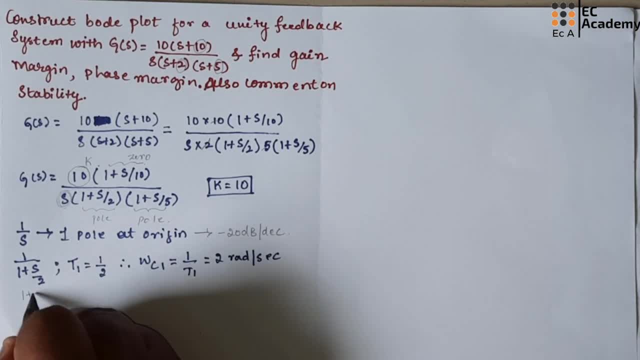 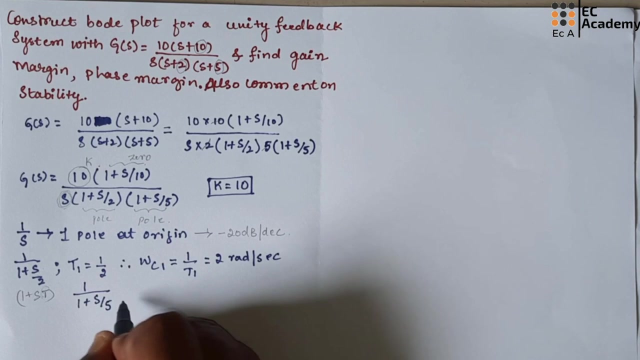 written this. we have compared this equation with 1 plus s, t. so if you compare these two terms, so here t can be written as 1 by 2. so in the same way for the next term, 1 by 1 plus s by 5. so we can. 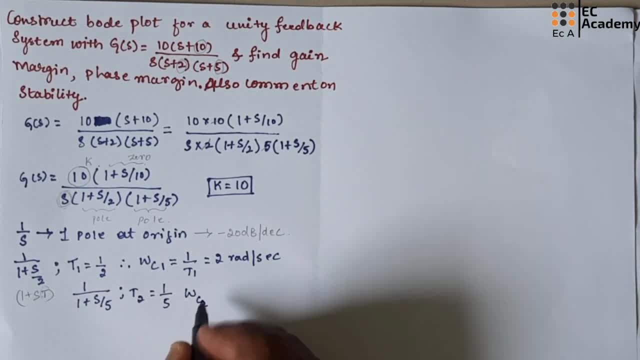 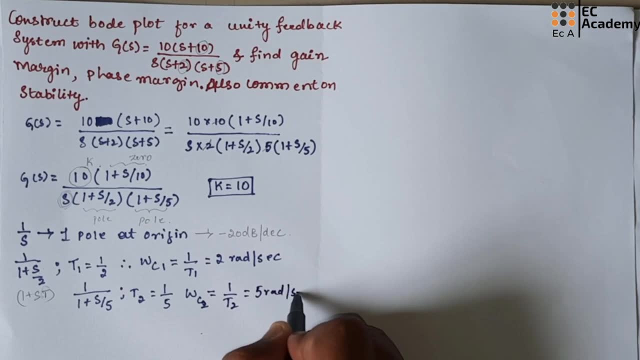 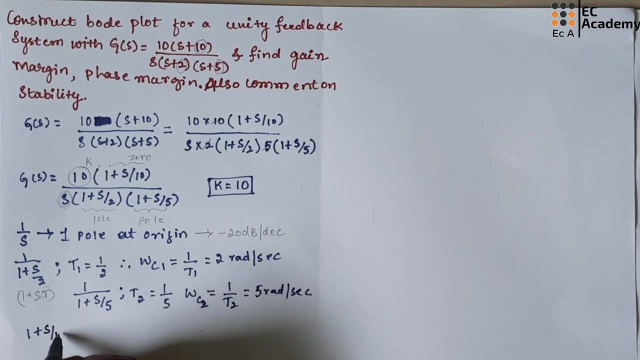 write, t2 is equal to 1 by 5. so second corner frequency, omega c2 can be written as 1 by t2. that is nothing but 5 radians per second. so we can take the numerator term which is 1 plus s by 10. so again, if we compare with the standard equation, so at that case we will get. 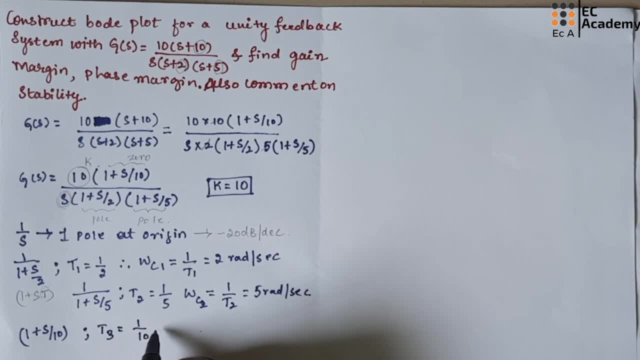 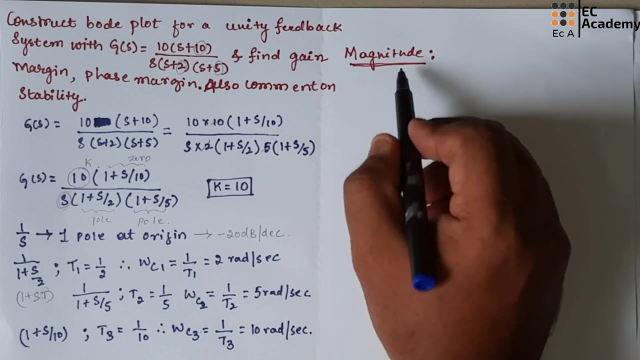 t3 is equal to 1 by 10. therefore we can write third corner frequency as 1 by t3. that is equal to 10 radians per second. now let us do the magnitude plot calculations in magnitude plot calculation. first we need to take: k is equal to 10 for that. 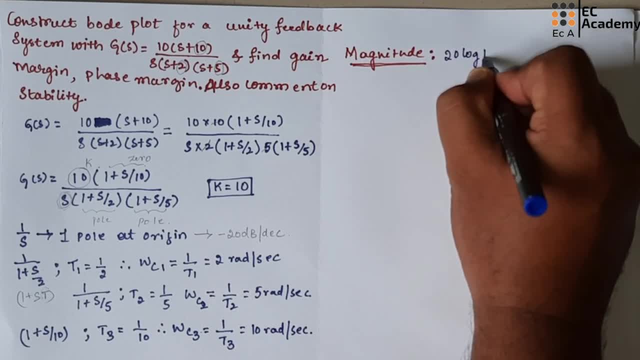 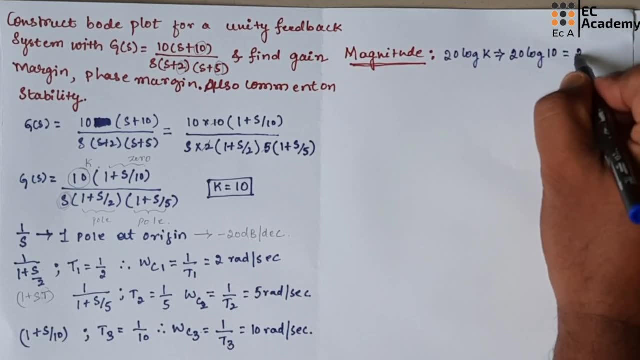 we need to find 20 log k, so, which means we need to find 20 log 10, so this value will be equal to 20 db per degree per decade. so we obtain 20 log k as 20 db per decade. so this 20 db per decade will be the. 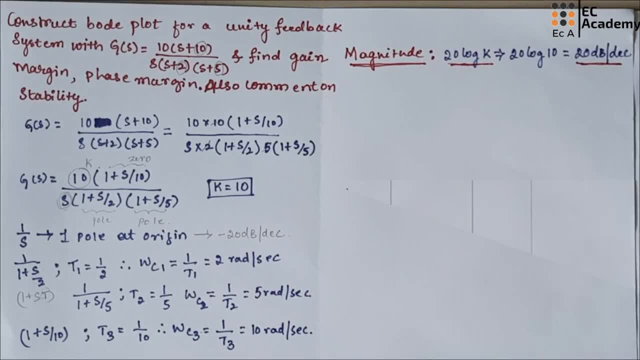 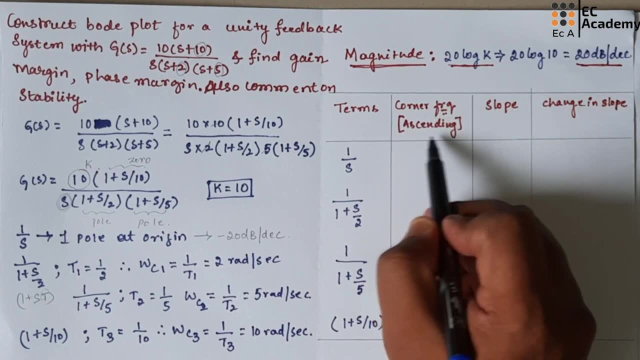 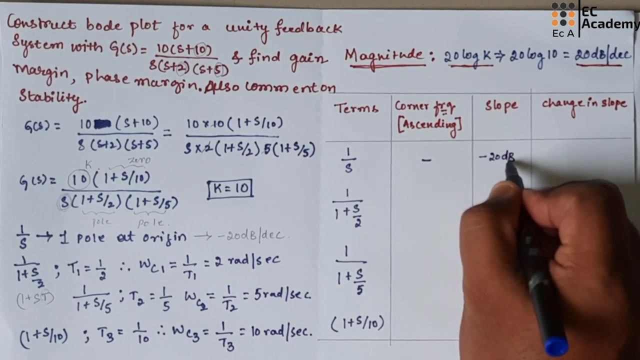 reference line in the magnitude plot. now we need to calculate the change in slope by considering term corner frequencies in ascending order slope and change in slope with respect to 1 by s. there will be no corner frequency since s is in the denominator. there will be a slope of minus 20 db per decade. so if there is s square in the denominator, 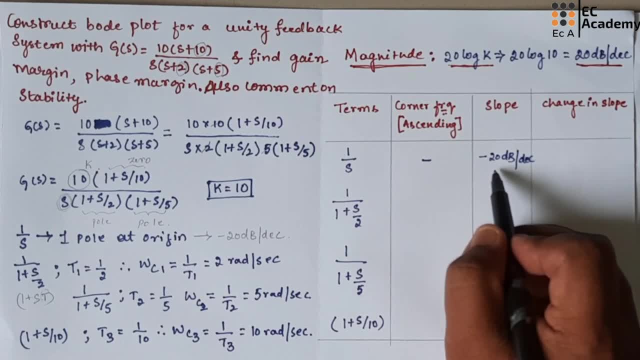 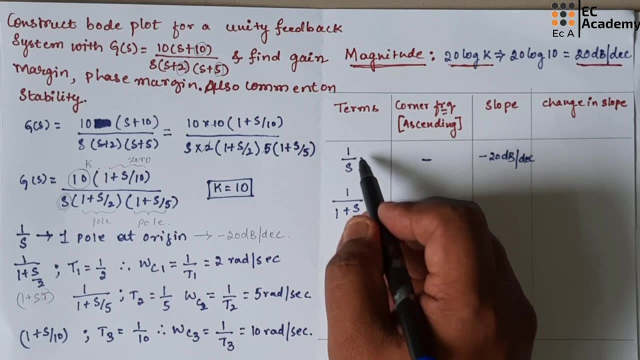 at that case we would have got the slope as minus 40 db per decade. so you can remember this for other problems. if s is in numerator, at that case we will get plus 20 db as slope, and if s square is in numerator, at that case we will get 40 db as slope. now, since it is, 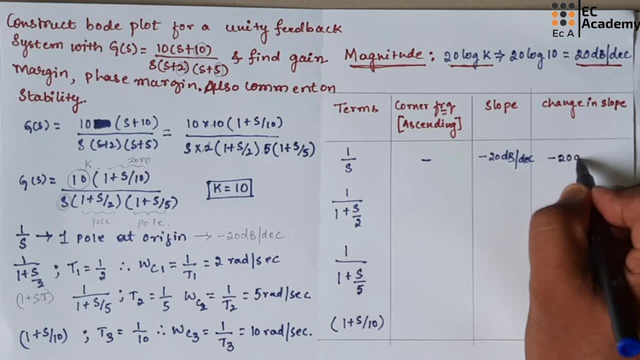 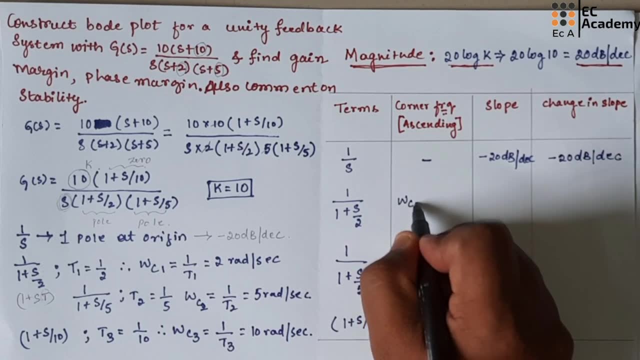 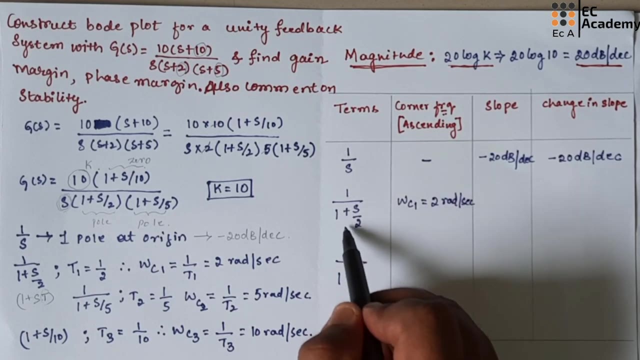 a first term, we will not have any change in slope. it will be minus 20 db per decade. now for the second term, we are having the corner frequency, as omega c1 is equal to 2 radians per second. again, here s is in the denominator. so that's why we will be having minus 20 db per decade. as 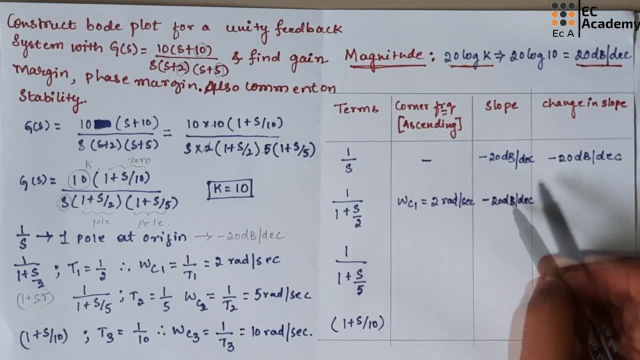 slope. now change in slope will be addition of these two slope values, so it will be minus 40 db per decade. now change in slope will be addition of these two slope values, so it will be minus 40 db per decade. now change in slope will be addition of these two slope values, so it will be minus 40 db per decade.